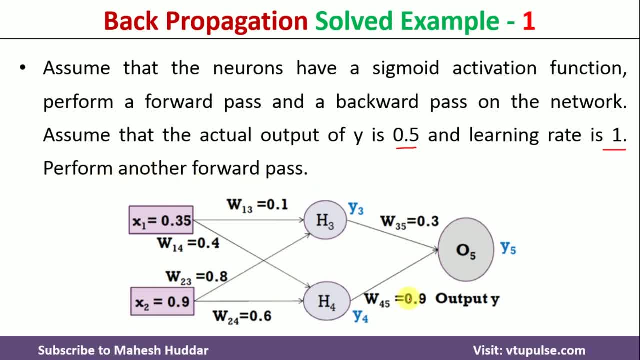 That is nothing but perform another forward pass here. Similarly, we have to do this particular steps again and again, unless and until we are happy with the error. So what we get at the output layer here, But in this case I am going to show it for two times. 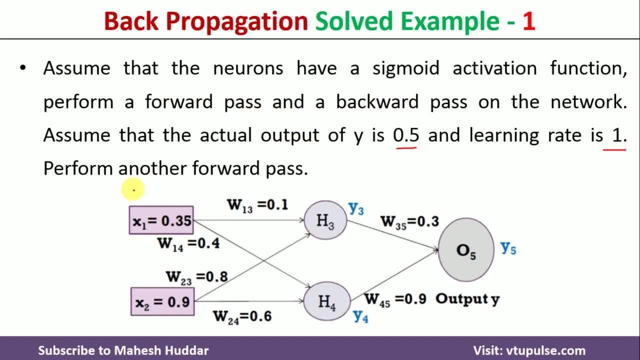 One time I will propagate the input, I will update the weights and then I will propagate the input through this particular network one more time. So that is two times. I will show here Now we will try to propagate this input through the network. 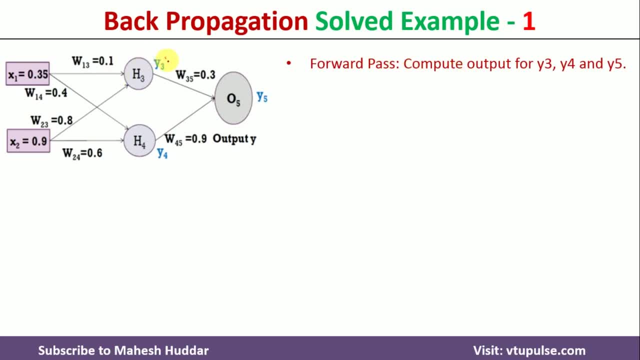 That is the forward pass here. For that reason we need to calculate this y3, y4 first, And then these y3 and y4 are the inputs, The inputs to this particular O5, again, we will calculate y5 here. 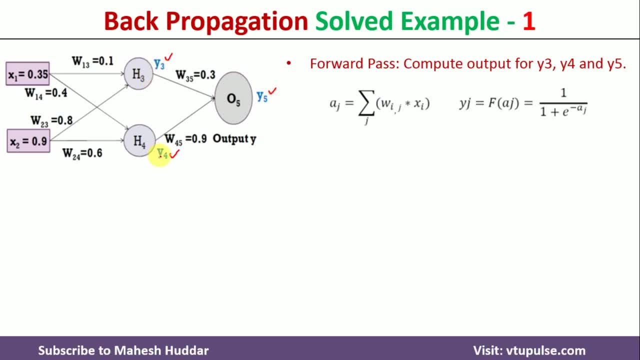 To calculate this y3 and y4, first we need to calculate what is that called as the summation term. That is nothing but Wij multiplied by xi. Once you calculate this particular summation term, we need to apply the activation function so that I will get this particular y3 and y4. 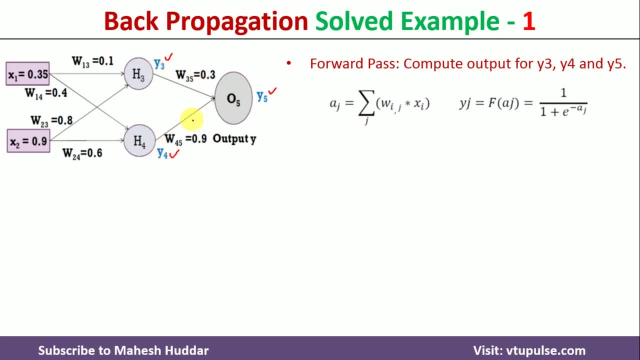 Similarly, we need to give this y3 and y4 as the input to here, And then we need to calculate the summation term, And then again we need to apply the activation function so that I will get the wi-fi here. Now, what is the activation function I am going to use? 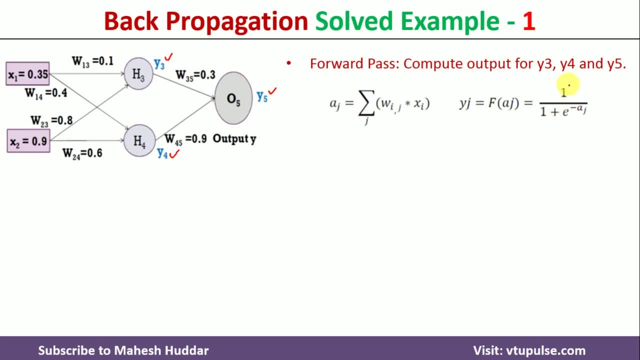 I am going to use the activation function as the sigma term. That is nothing but 1 divided by 1 plus e raise to minus x. In this case I am calculating aj. Hence it is minus aj here. So first we will calculate the value of aj. 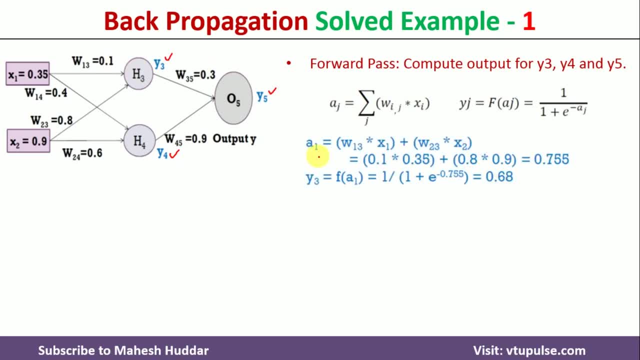 That is the summation term at h3.. That is nothing but a1. here a1 is equal to W13 multiplied by x1 plus W23 multiplied by x2.. So that is the term over here. So if I put those particular values, I will get 0.755. 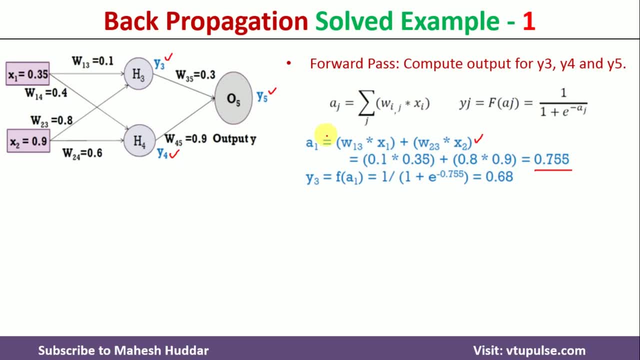 That is, W13 is 0.1, x1 is 0.35.. That is the term over here. Similarly, 0.8 is W23 and x2 is 0.9.. So that is what I have written here. 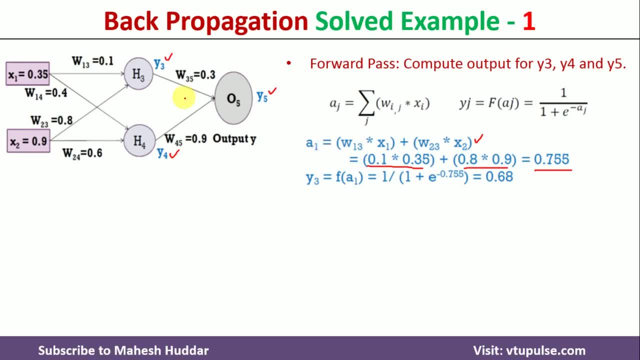 Now, once you get this particular a1, I have to apply the activation function so that I will get y3 here. y3 is equal to f, which is equal to 1 divided by 1 plus e raise to minus a1 here. 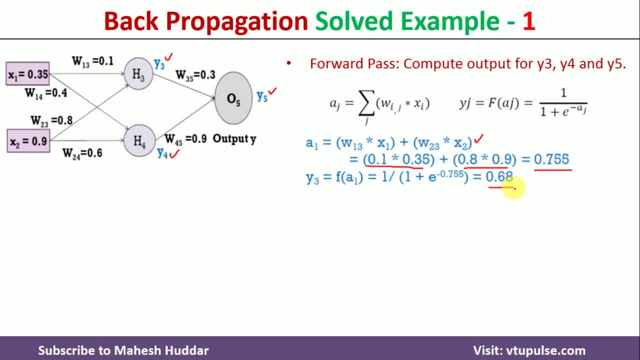 a1 value is 0.755.. I will get 0.68 in this case. So this is the output at h3 here. Similarly, I will calculate the output at h4.. That is nothing, but a2 is equal to. 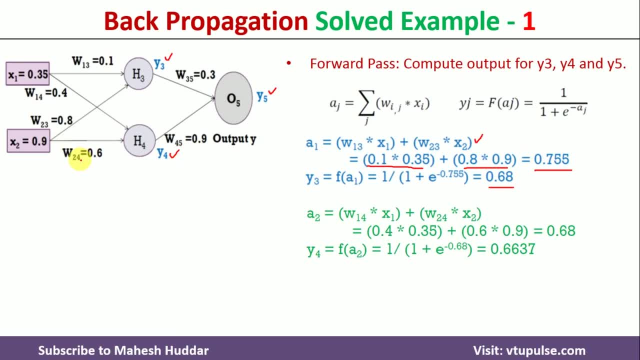 W14 multiplied by x1, plus W24 multiplied by x2.. So that is what I have written here, And then I will put the values. I will get a2 as 0.68.. I will calculate the y4 by applying activation function here. 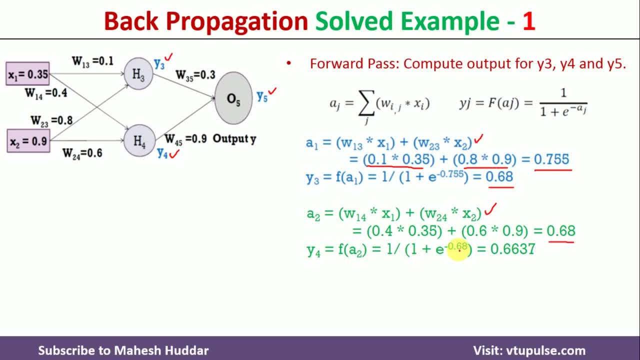 y4 is equal to 1 divided by 1 plus e raise to minus a2.. That is 0.68.. I will get 0.6637 here. So I got the value of y3.. I got the value of y4 here. 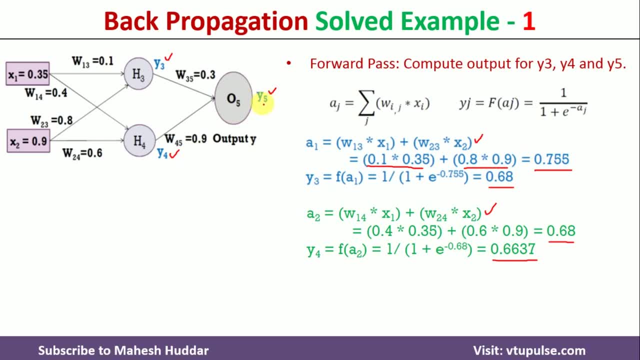 I will give this as an input to this o5 and then calculate y5 here. So if I want to calculate the y5, first I will calculate a3. here a3 is nothing but W35 multiplied by y3 plus W45 multiplied by y4 here. 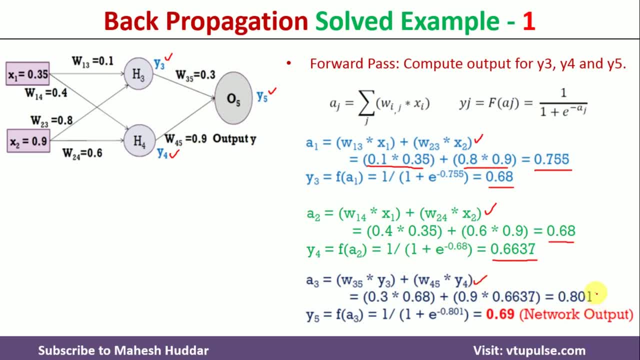 So I will put all those particular values here. I will get 0.801 as the a3.. Now I will put this particular a3 or I will pass a3. as to the activation function, I will get y5 here. 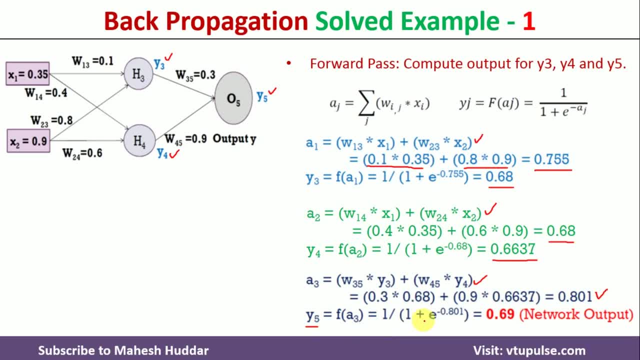 y5 is equal to f of a3. That is nothing but 1 divided by 1. plus e raise to minus a3.. a3 value is 0.801, which is equal to 0.69.. That is the output at the output unit here. 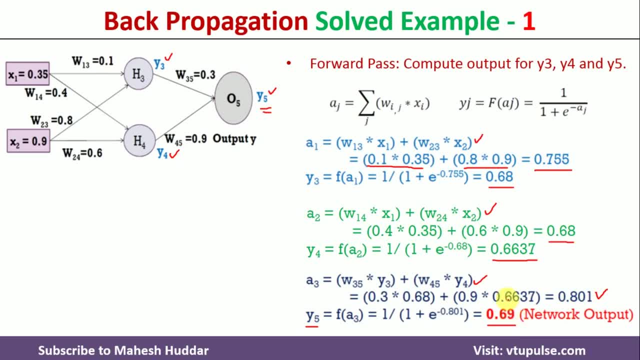 So the output at the output unit is 0.69.. Now what is the expected output? The expected output is 0.5, but I am getting 0.69.. So the error is equivalent to the expected is 0.5 here, but I am getting 0.69.. 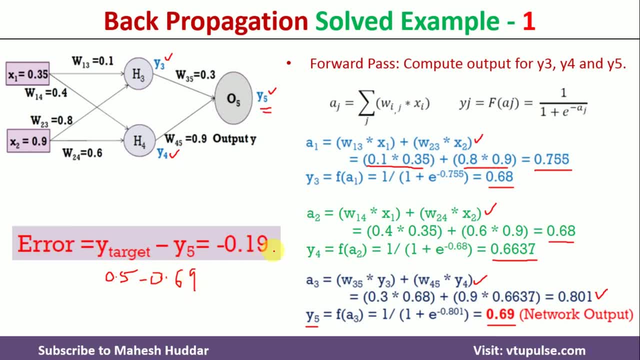 So the error will be in this case, we can say that minus 0.19 in this case. So this is how actually we can propagate the input through the network and then we calculate the error here. Now, once you calculate this error, we have to cross check whether I am happy with the error or not. 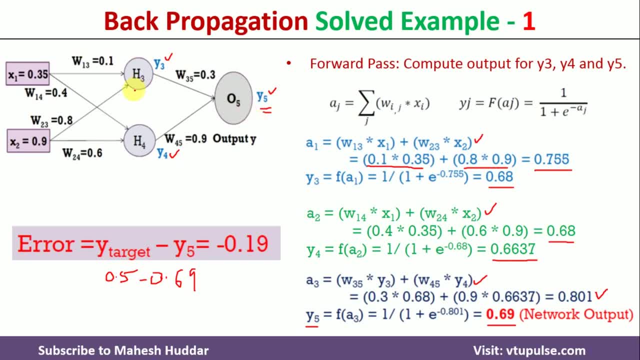 If it is not, we have to update this particular weights. In this case, I will try to update the weights and then I will try to show how can we reduce this particular error over here. Now. if I want to update the weights, we have to use this particular equation. 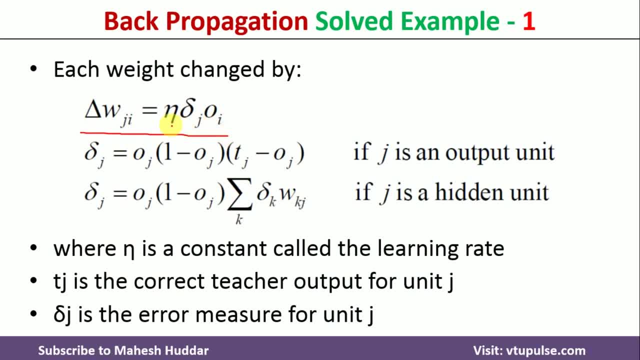 That is delta wji is equivalent to n. that is the learning rate multiplied by delta j. that is the error term at jth unit. oi is nothing but the output at ith unit. Now, how to calculate this particular delta j? Because we know the value of the learning rate, that is equivalent to 1 in this case. 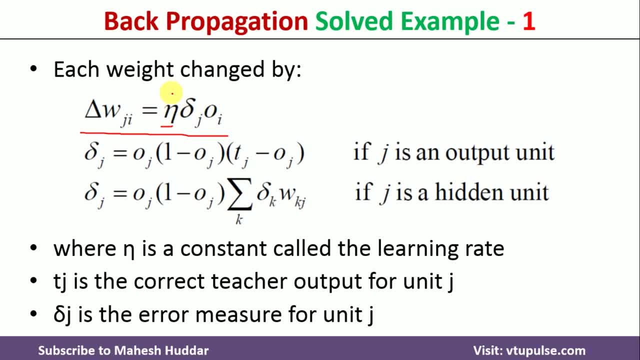 That is the constant value we can consider for a given problem. But delta j is the error at the jth unit, So we have to calculate it. So there are two kind of units are there In this case. we can see here these two, h3 and h4, are the hidden units. 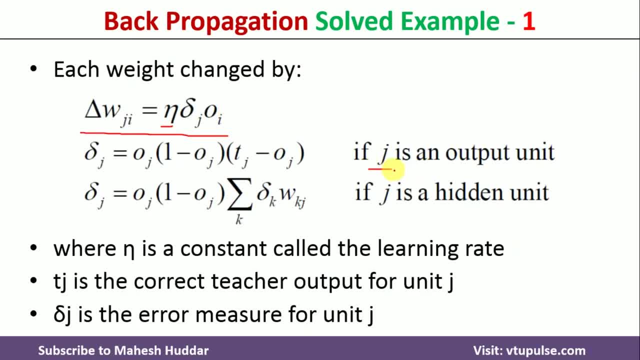 o5 is the output in it. So if the j is the output in it, the delta j is equivalent to 0.. oj multiplied by 1 minus oj, multiplied by tj minus oj, That is the output at jth unit multiplied by 1 minus output at jth unit, multiplied by target minus the calculated output at the jth unit. 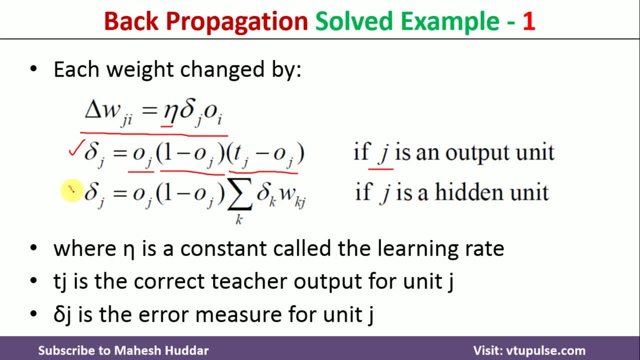 Similarly, if j is the hidden unit, we need to use this equation, That is, delta j is equivalent to, again, oj multiplied by 1 minus oj, But summation of delta k multiplied by wkj, Where k is the number of output units. in this case. 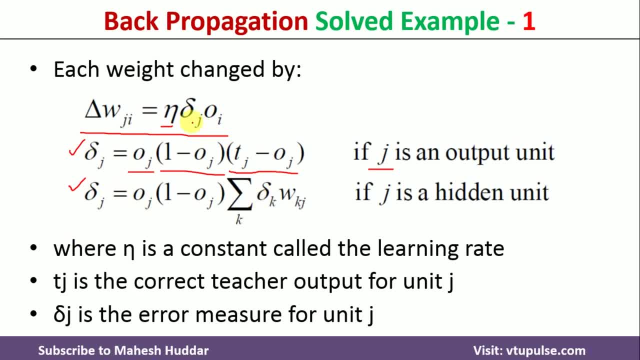 So, using these particular equations, we calculate the delta j term. We have already calculated the output at each unit. Using those three, we will calculate the modified weight in this case. So first we will try to calculate the delta term at each and every unit. 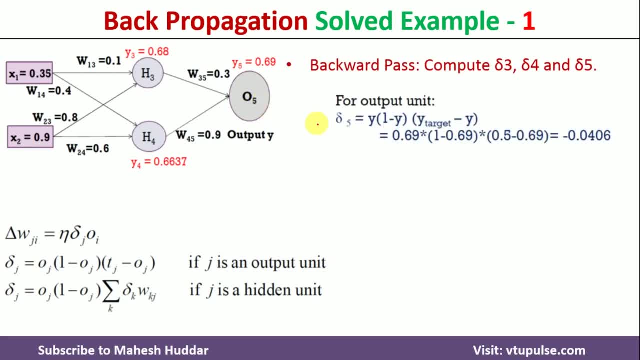 So first we calculate the delta term at the output in it, That is delta 5.. Because it is the output in it Which is equivalent to y minus 1 minus y, That is the calculated output multiplied by 1 minus calculated output. multiplied by what is the value we have here? 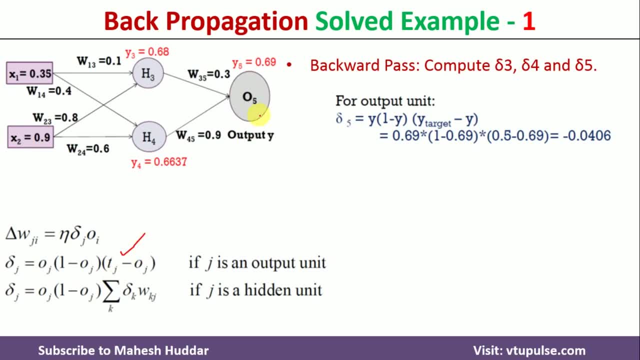 This is tj minus oj. tj is what The target output, That is 0.5, what we are expecting, and y is the calculated output. So what is the calculated output in this case is 0.69.. 1 minus 0.69.. 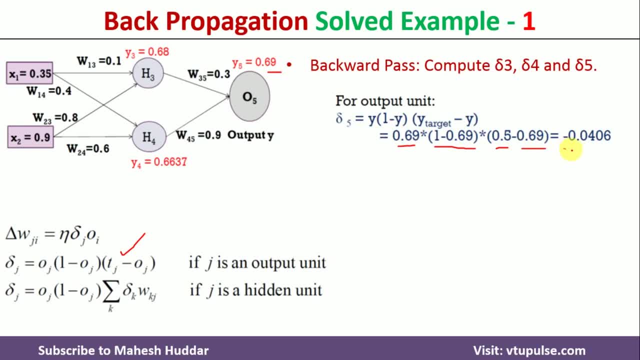 0.5 is the target, 0.69 is the calculated output. Hence delta 5 is equivalent to minus 0.0406 here. Now we will try to understand how to calculate the error term at h3 here. 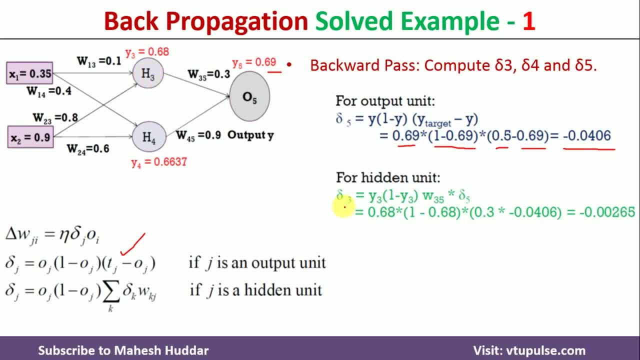 So if you want to calculate error at h3, the equation is: we have to use this one. the second equation, That is, delta 3, is equivalent to y3 multiplied by 1 minus y3.. That is the calculated output at h3 multiplied by 1 minus y3. 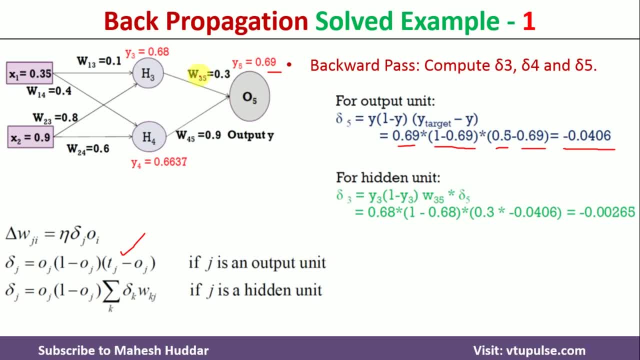 Multiplied by this weight, that is w35, and the error calculated at the output in it, that is delta 5.. Because we have only one output in it, we get the summation term as only 1. If we have multiple number of output in it, I will get the summation here. 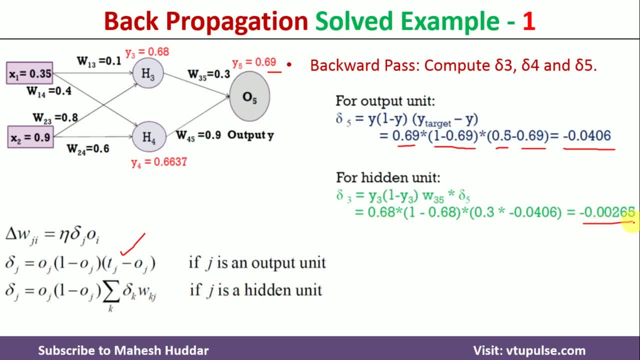 I will put all the values here. I will get the answer as minus 0.00265.. Similarly, I will calculate the error term at h4 also. That is, delta 4 is equivalent to y4 minus 0.00265.. 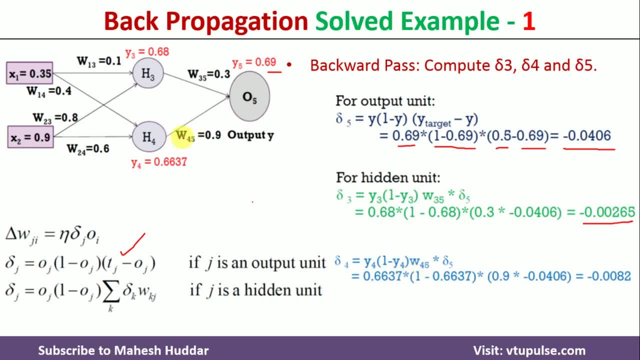 Multiplied by 1 minus y4.. Multiplied by this weight and the error at this particular output in it, That is 0.9. multiplied by this we have already calculated. I will put it over here. So the total answer in this case is minus 0.0082 here. 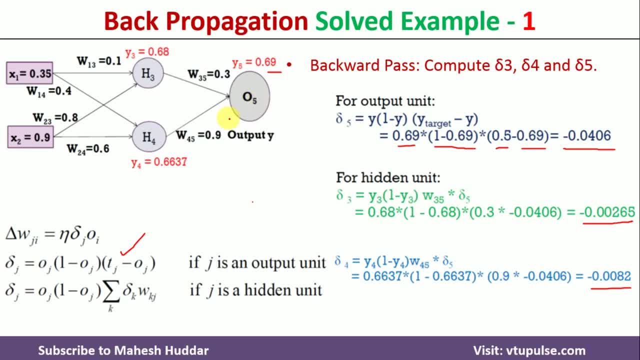 So what we did is we calculated error at the output. in it We calculated the error at the hidden units. So using this thing, we have to modify this particular weights here, That is, delta wj is equivalent to learning rate multiplied by delta j. 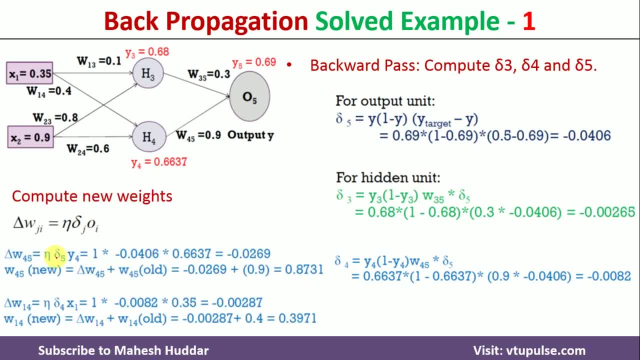 That is delta wj multiplied by oi here. So what I do here is I will put the calculated values. I will show one example. That is w45.. Delta w45 is equivalent to n multiplied by delta 5 y4, which is equivalent to minus 0.0269. 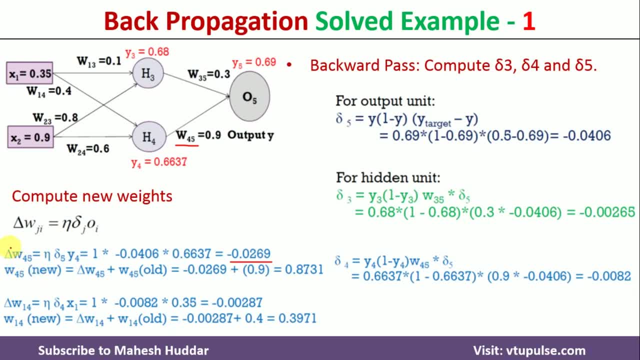 Similarly, we will calculate one more. This is the delta term. actually, This is not the final term. So what we do is we will add this thing to the previous weight. What is the previous weight here? 0.9.. 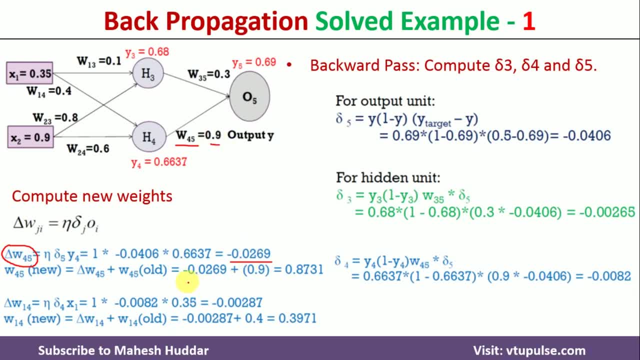 So to this particular previous weight we will add this particular the delta term. If I add it, I will get this particular thing. That is nothing but the modified weight here. Similarly, I will show one more, That is w14.. 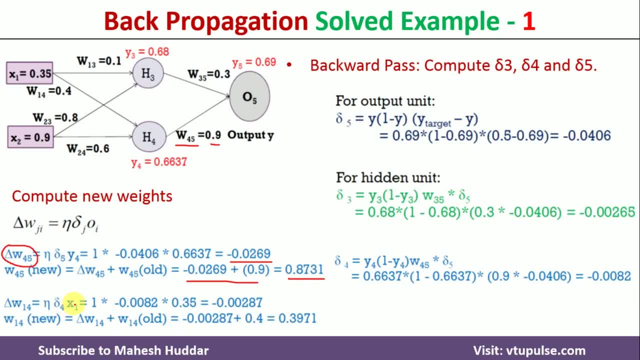 w14 is equivalent to n multiplied by delta 4 x1.. That is, 1 multiplied by the delta 4.. The delta 4, we know that value, Delta 4, somewhere we have calculated it. This is the delta 4 value multiplied by 0.35. 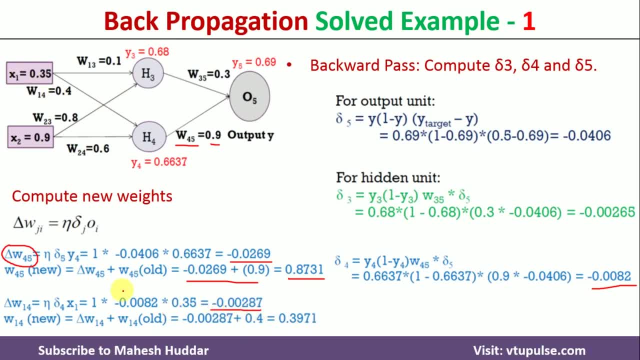 That is x1.. The delta term. what we get here is, or we can say that the increment or decrement we will get is minus 0.00287.. Once you add it to the old value, I will get the modified weight here. So this is the modified weight. 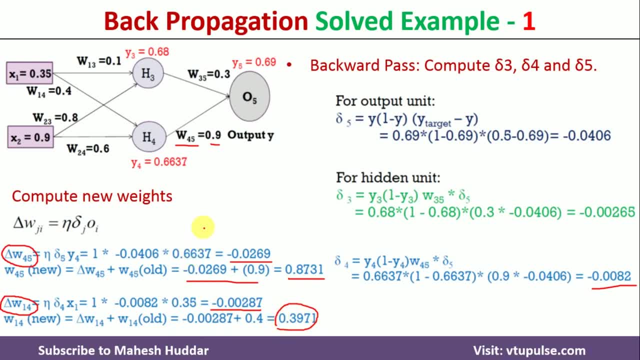 So this is how actually we can calculate the modified weights. in this case I have shown two: This 0.9 is modified to 0.8731 and this 0.4 is modified to 0.3971 in this iteration. 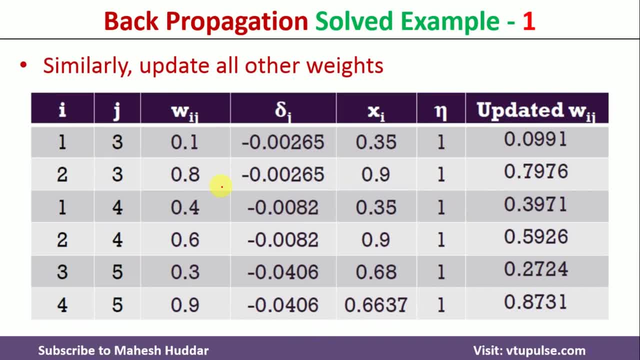 Similarly we have to calculate all the modified weights here. So once you calculate this particular modified weights, you can see here wji is calculated for every combination. and then we have got this particular updated wji by adding this particular delta wji to this. 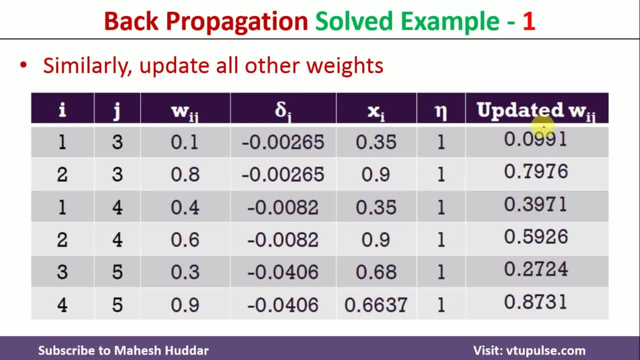 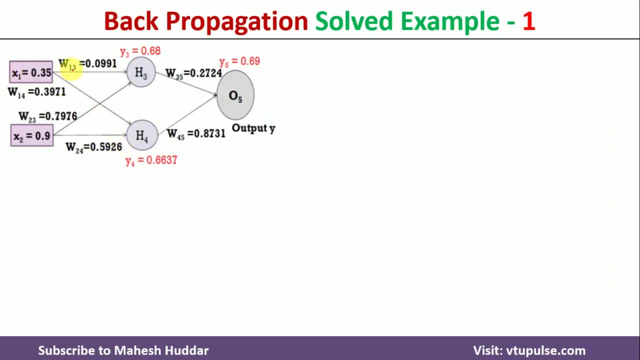 This is the old value. Now, once you get this particular updated values for all the weights, the network looks something like this. You can see here: w13 is equal to 0.0991.. w24 is equal to 0.5926, and so on. 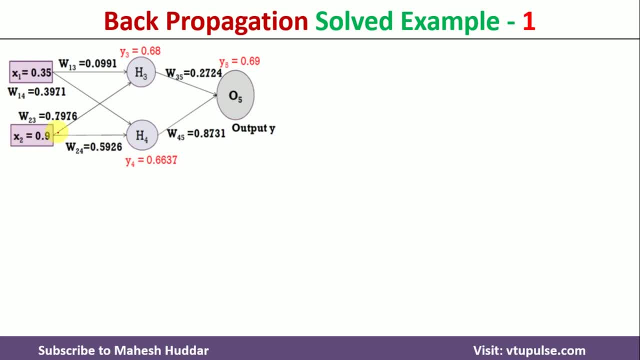 Again, we need to pass this particular x1 and x2 forward through this network and then we need to calculate the output. If the output is correct or acceptable, we can stop here. Otherwise we need to use the same process, like calculating the error at each neuron. 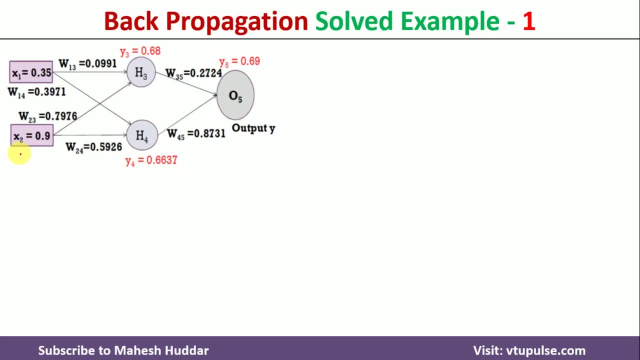 updating the weights and then passing this particular input forward through this network. The same process has to be followed again and again in this case. So first what we do is we try to calculate what is y3, y4 and y5.. y3, if you want to calculate, first we need to calculate the summation term, and then we need to apply this activation function again here. 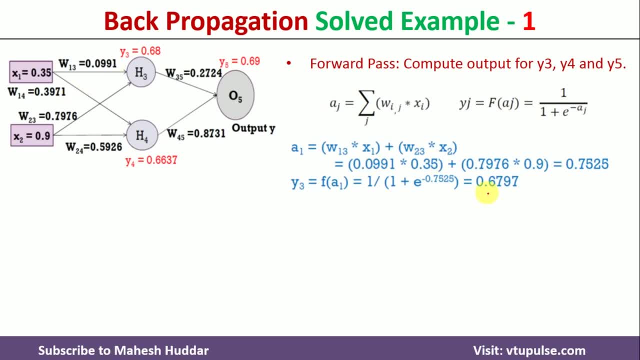 So we have this value. So we calculate it Now. y3 is 0.6797.. So previous value was 0.68.. Now it is modified to 0.6797.. Similarly we calculate the y4..